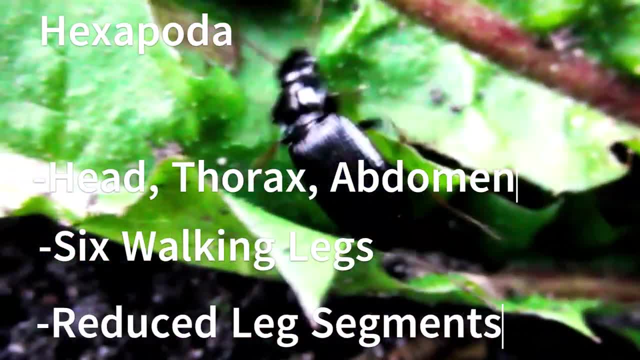 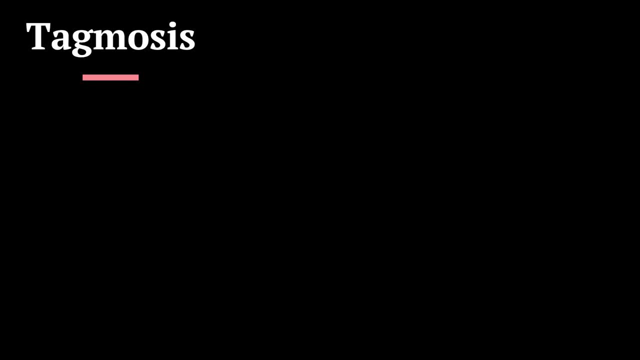 hexapod comes from, as well as a reduced number of leg segments. The segmentation of the insect body into three distinct regions is a result of a process known as tagmosis. Tagmosis is the fusion of body segments into specialized regions known as tagmata. Six legs are divided into three pairs. 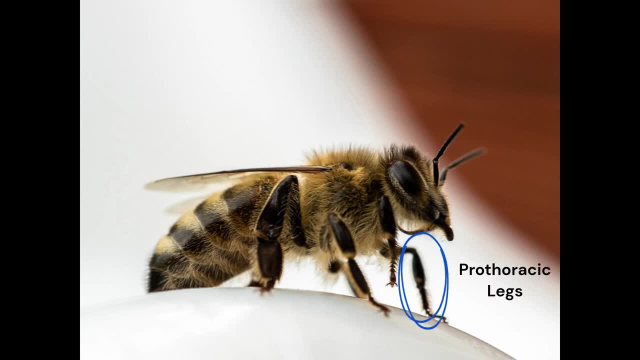 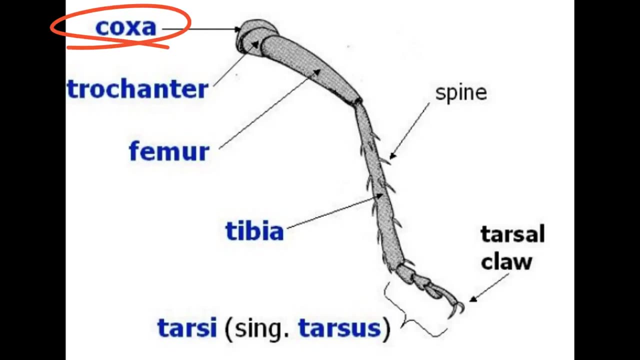 ordering from head to abdomen. These legs are referred to as the prothoracic legs, the mesothoracic legs and the metathoracic legs. The insect leg is divided into five parts, known as the coxa, the trochanter, the femur, the tibia and the tarsus, or tarsal claw. 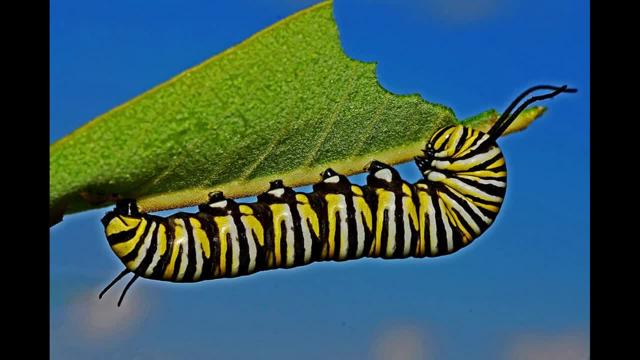 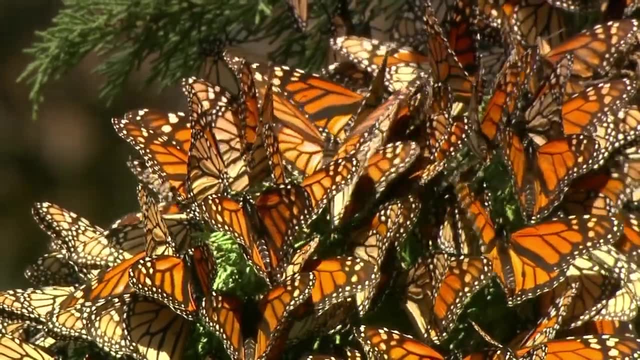 Larvae of some insects such as caterpillars have many smaller leg protrusions, called prolegs, that aid in grip and movement. Some characteristics are notable of hexapods but do not represent the entire group. These include structures like wings and antenna. This is because only certain insects have wings and may not have wings. The legs are divided into five parts known as the coxa, the tarsal claw, the femur, the tarsal claw and the tarsal claw. Many other types of arthropods have. 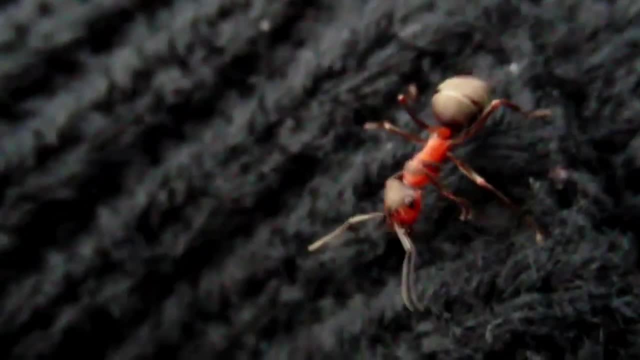 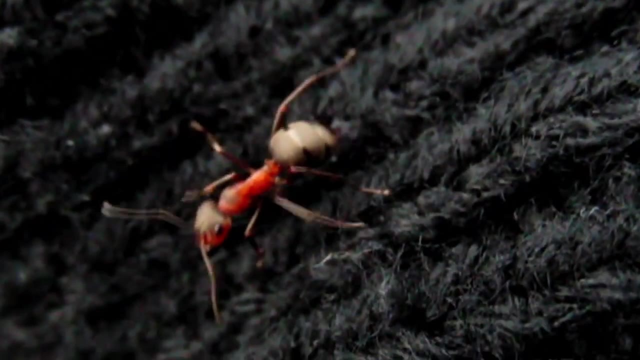 antenna. By far the most successful group of both hexapods and all arthropods in general are the insects. There are a few key reasons why the insects became such a successful group, and they are as follows. The first reason that insects became so successful is due to the leg up they've 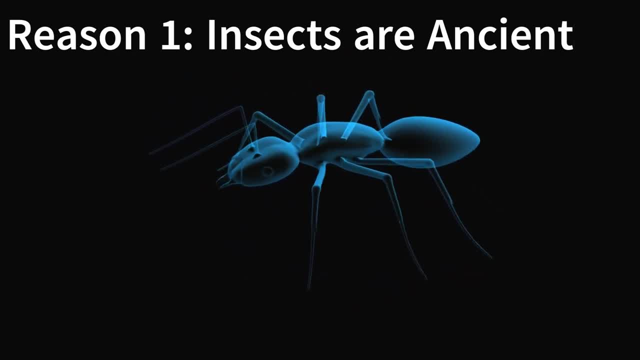 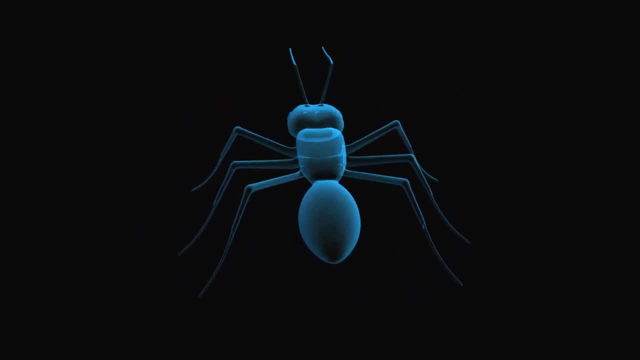 had in terms of evolution, with their ancestors colonizing land 400 million years ago, 25 million years before vertebrates. This allowed the insects to diversify rapidly before other groups of animals could. The second reason insects have been so successful is due to their hardiness when it comes to extinction. 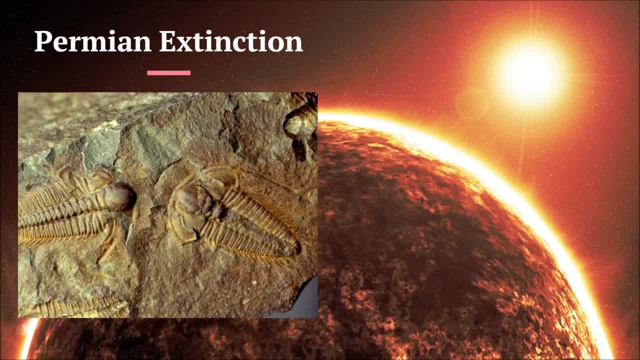 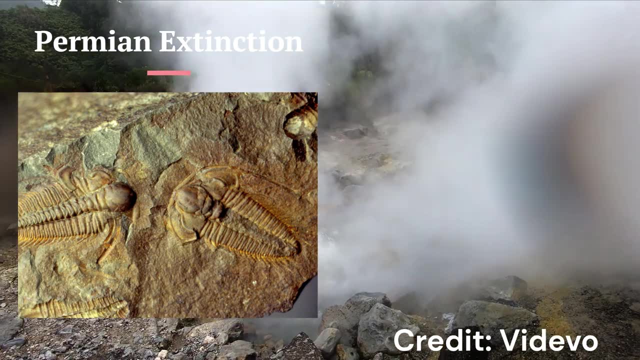 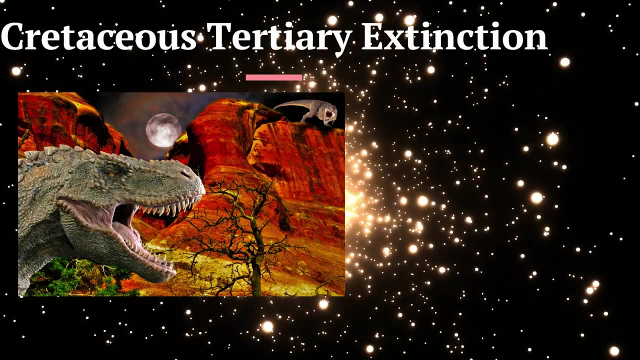 events During the end Permian event, an extinction event. around 252 million years ago, over 95% of marine organisms went extinct, whereas the main terrestrial organisms at the time- the insects, only lost around 55% of all species. In addition, during the Cretaceous-Tertiary extinction, 65. 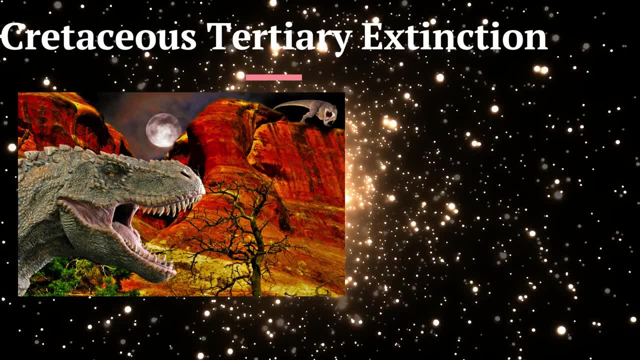 million years ago, 50% of all species went extinct. However, insect numbers were relatively unaltered. The third reason insects have been so successful is due to their hardiness when it comes to extinction events. This allowed the insects to diversify rapidly before other groups of animals could.